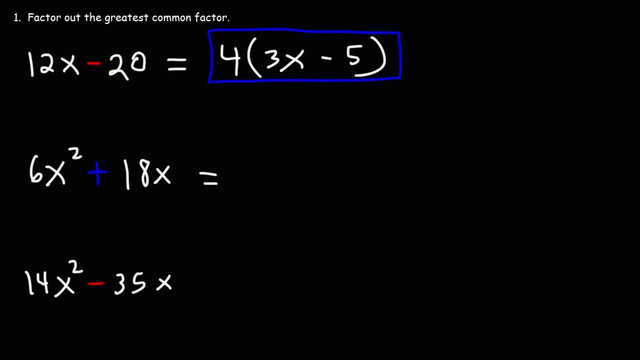 So what is the greatest common factor? that we can take out 6 and 8, I mean 6 and 18, they're both multiples of 6. So we can take out a 6.. Now, both of these terms contain at least one x variable. 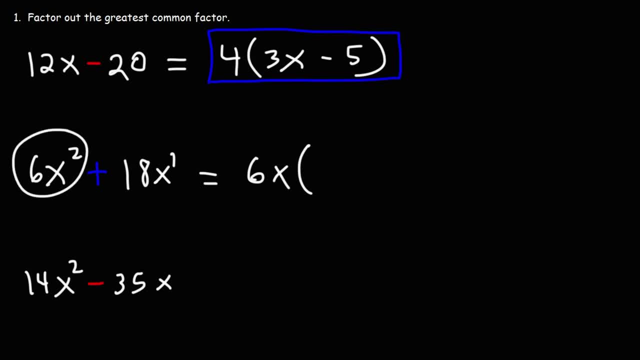 So we can take out an x. Each of these terms are divisible by 6x. 6x squared divided by 6x is x. 18x divided by 6x is positive 3.. So this is the answer. It's 6x times x plus 3.. 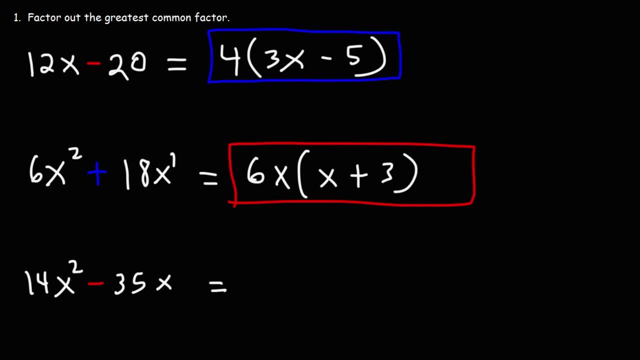 Now, what is the GCF for the next one? 14 and 35 are multiples of 6x, So we can take out a 6x, 7 can go into 14 and 35.. Here we have an x squared, Here's an x. 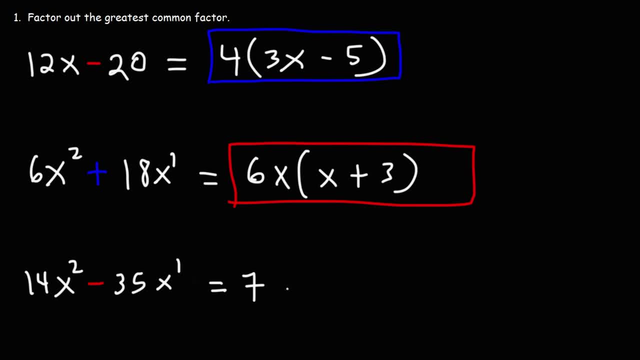 So we can take out at least one x out of the two. So the GCF is 7x 14x squared. divided by 7x, that's going to be 2x Negative. 35x divided by 7x, that's going to be negative 5.. 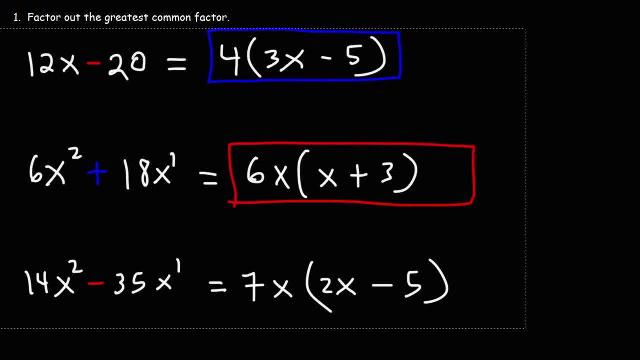 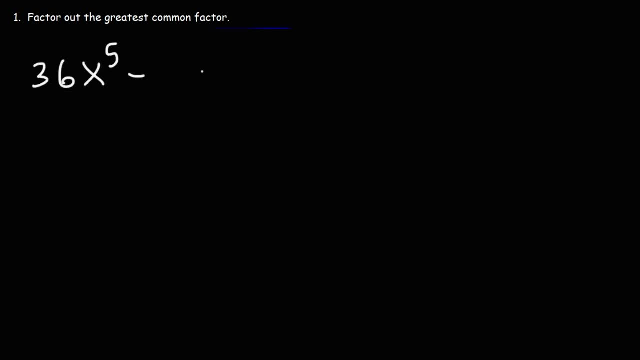 So that's the answer. Let's try another similar example. So let's say we have 36x to the 5 minus 63x cubed. What's the GCF in this case? The highest multiple? I'm 36 and 63.. 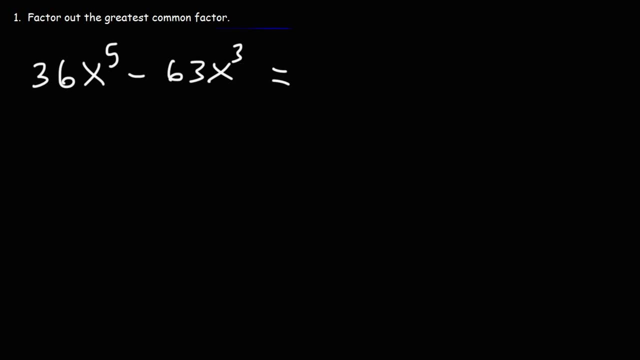 What is the highest number that goes into both. Both of those numbers are divisible by 3 and they're divisible by 9.. So 9 is going to be part of the GCF. Now, looking at these two, the smaller of them is x cubed. 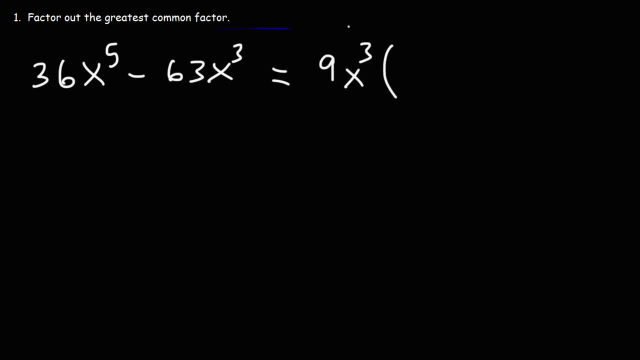 So x cubed is going to be part of the greatest common factor. Now, if we take 36x to the 5th power and divide it by our GCF, this is going to be 36 divided by 9 is 4.. 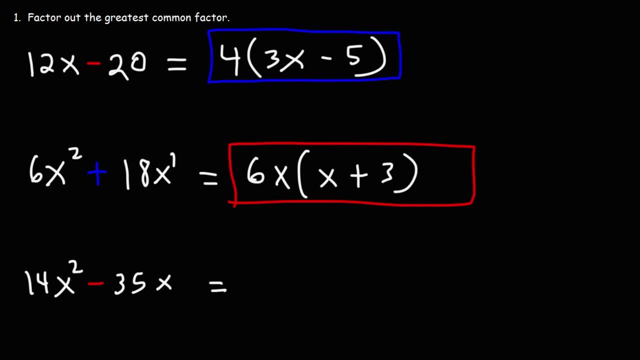 Now, what is the GCF for the next one? 14 and 35 are multiples of 6x, So we can take out a 6x, 7 can go into 14 and 35.. Here we have an x squared, Here's an x. 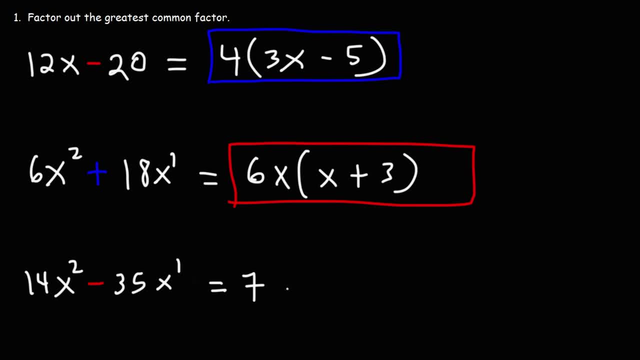 So we can take out at least one x out of the two. So the GCF is 7x 14x squared. divided by 7x, that's going to be 2x Negative. 35x divided by 7x, that's going to be negative 5.. 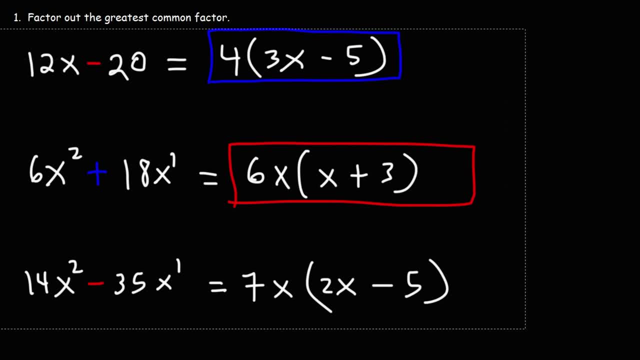 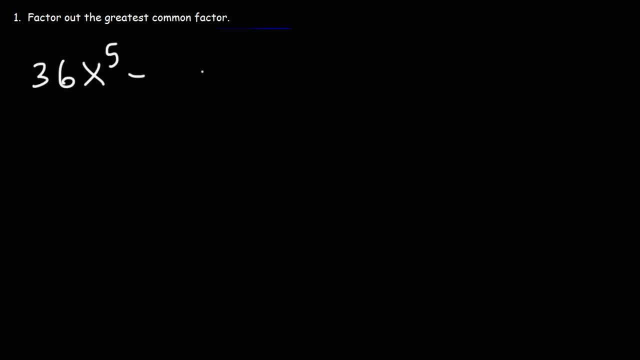 So that's the answer. Let's try another similar example. So let's say we have 36x to the 5 minus 63x cubed. What's the GCF in this case? The highest multiple? I'm 36 and 63.. 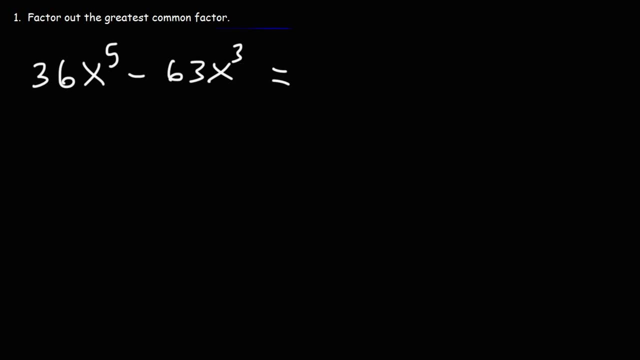 What is the highest number that goes into both. Both of those numbers are divisible by 3 and they're divisible by 9.. So 9 is going to be part of the GCF. Now, looking at these two, the smaller of them is x cubed. 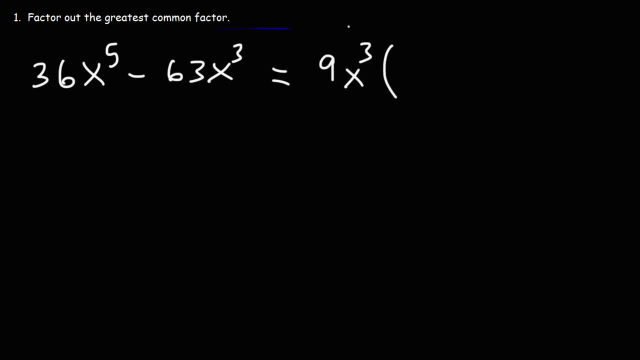 So x cubed is going to be part of the greatest common factor. Now, if we take 36x to the 5th power and divide it by our GCF, this is going to be 36 divided by 9 is 4.. 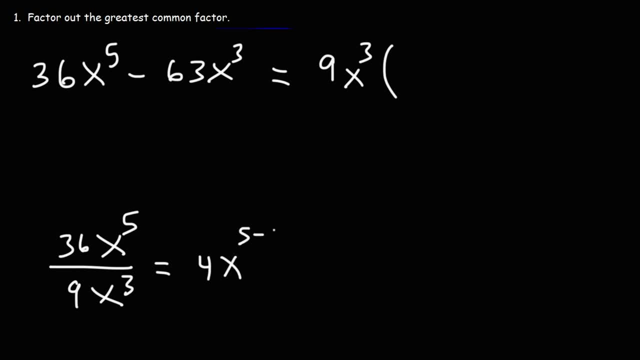 x to the 5 divided by x, cubed, we need to subtract the exponents, So we're going to get 4x squared. That's going to go in here. Next we need to divide this by the GCF to get the next term inside the parentheses. 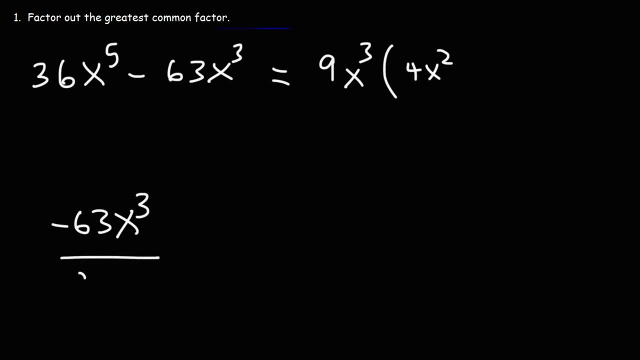 So if we take negative 63x cubed and divide it by the GCF, these two will cancel. So negative 63 divided by 9 is negative 7.. So we're going to have a minus 7 inside here. So that's how we can factor out the greatest common factor in these problems. 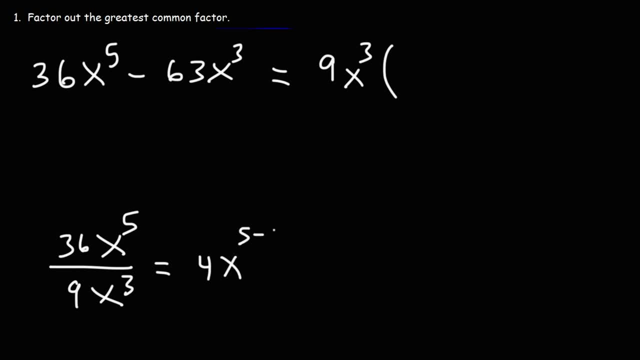 x to the 5 divided by x, cubed, we need to subtract the exponents, So we're going to get 4x squared. That's going to go in here. Next we need to divide this by the GCF to get the next term inside the parentheses. 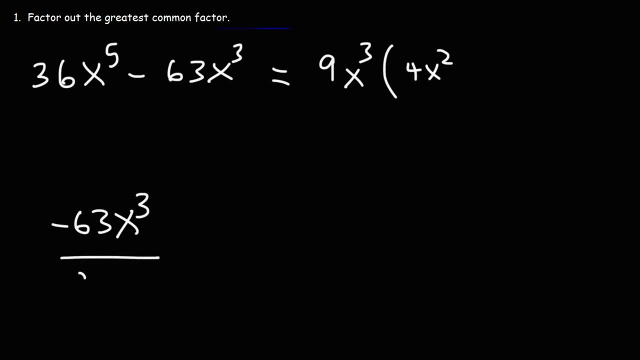 So if we take negative 63x cubed and divide it by the GCF, these two will cancel. So negative 63 divided by 9 is negative 7.. So we're going to have a minus 7 inside here. So that's how we can factor out the greatest common factor in these problems. 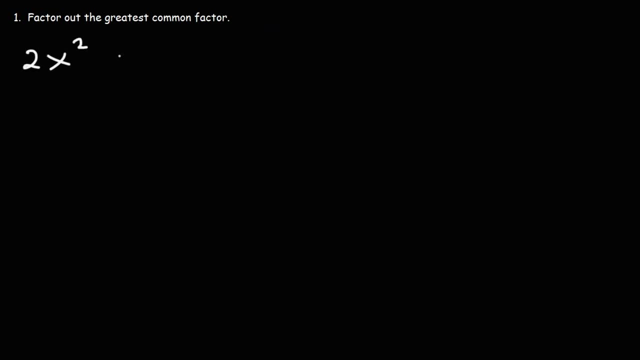 Now let's move on to the next example. Try these two problems. Let's say we have 2x squared Minus 8x plus 10. And also 27x to the 5th power Plus 36x cubed. 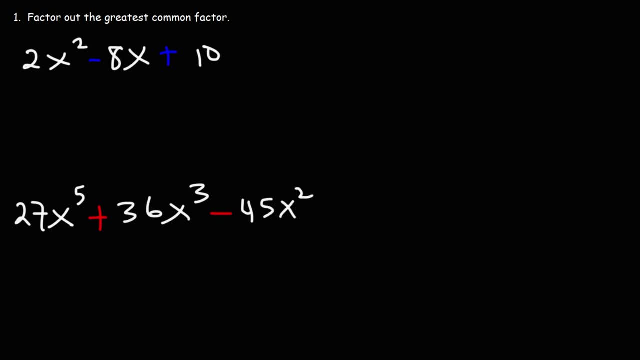 Minus 45x squared. So go ahead and factor these expressions by pulling out The GCF. So here we have a trinomial with three terms. What we can do is take out a, 2.. All of the coefficients are divisible by 2.. 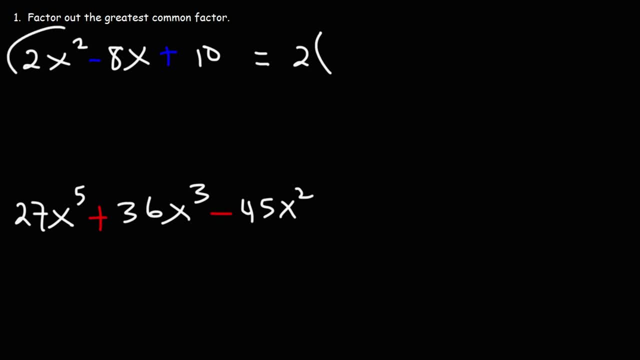 So that's going to be the GCF. the greatest common factor: 2x squared divided by 2 is x squared Negative. 8x divided by 2 is negative 4x And 10 divided by 2 is 5.. 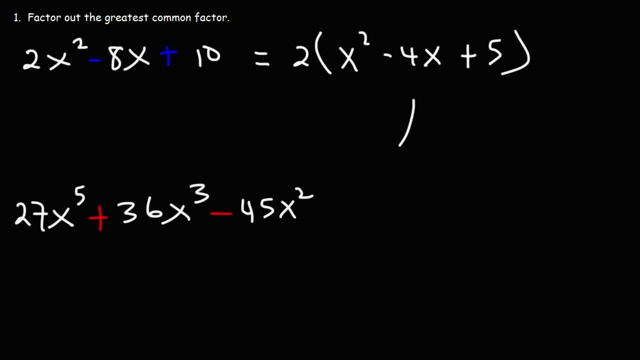 So we have a polynomial with three terms, which is called a trinomial. Now what can we do? at this point, It doesn't look like we can factor this trinomial, so we're going to leave it the way it is. 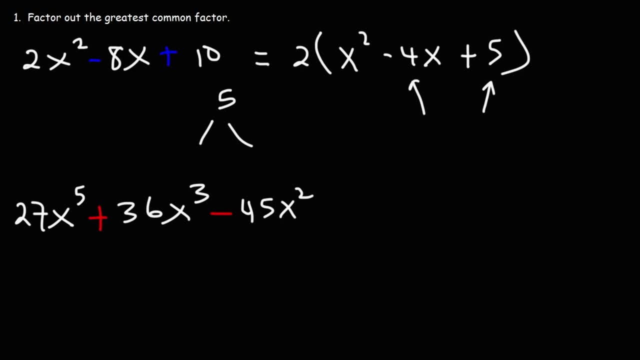 In order to factor it, we need to find two numbers that multiply to 5 but add to negative 4.. And that's not possible. Two numbers that multiply to positive 5 are negative 1 and negative 5, but they add up to negative 6.. 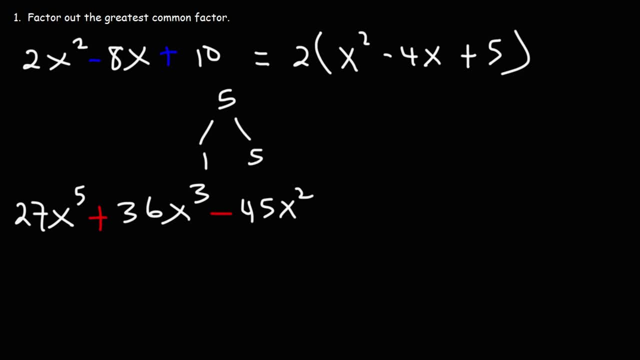 The other option, Positive 1 and positive 5, which adds the positive 6.. So we can't factor this trinomial. Therefore, we're going to have to leave the answer that way. Now for the next one. what is the GCF? 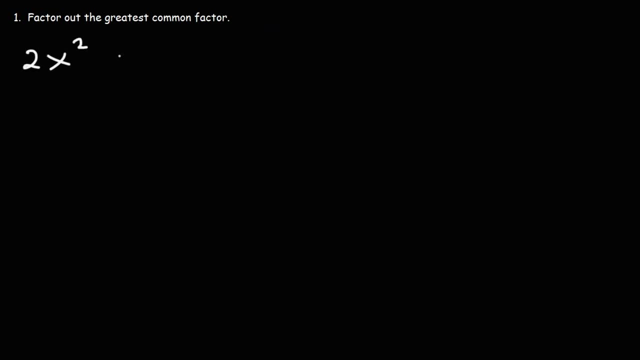 Now let's move on to the next example. Try these two problems. Let's say we have 2x squared Minus 8x plus 10. And also 27x to the 5th power Plus 36x cubed. 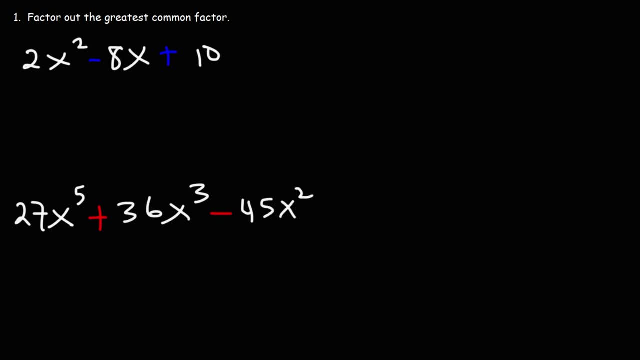 Minus 45x squared. So go ahead and factor these expressions by pulling out The GCF. So here we have a trinomial with three terms. What we can do is take out a, 2.. All of the coefficients are divisible by 2.. 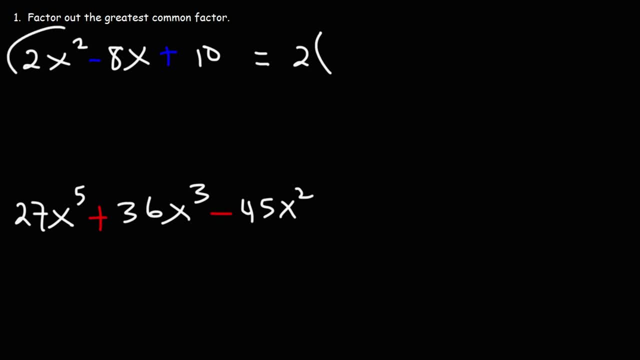 So that's going to be the GCF. the greatest common factor: 2x squared divided by 2 is x squared Negative. 8x divided by 2 is negative 4x And 10 divided by 2 is 5.. 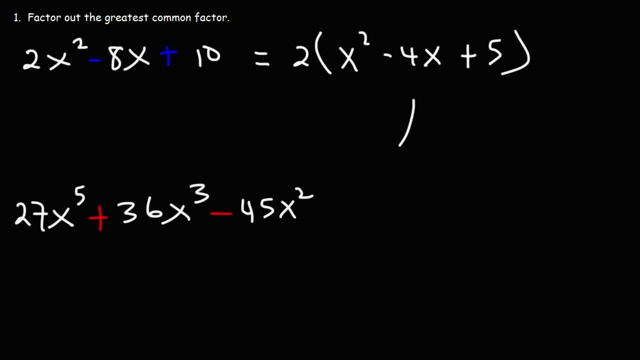 So we have a polynomial with three terms, which is called a trinomial. Now what can we do? at this point, It doesn't look like we can factor this trinomial, So we're going to leave it the way it is. 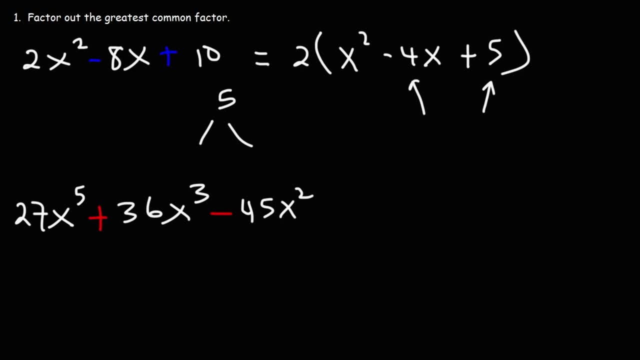 In order to factor it, we need to find two numbers that multiply to 5 but add to negative 4.. And that's not possible. Two numbers that multiply to positive 5 are negative 1 and negative 5. But they add up to negative 6.. 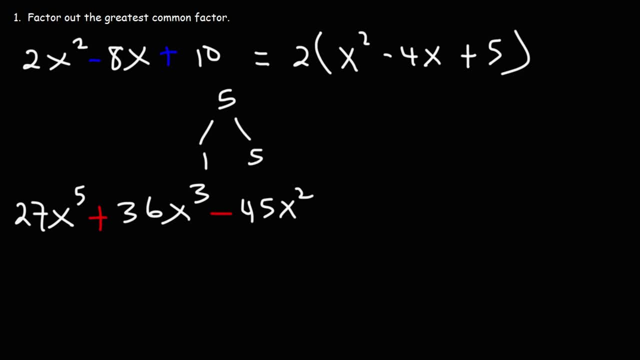 The other option Is positive 1 and positive 5, which adds the positive 6.. So we can't factor this trinomial. Therefore, we're going to have to leave the answer that way. Now for the next one. what is the GCF? 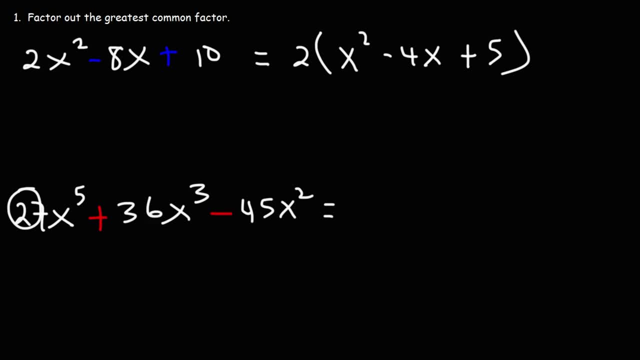 Notice that 27,, 36 and 45. They're divisible by 9.. And looking at the smaller of these three, it's going to be x squared, So we could factor out 9x, 27x to the 5th, divided by 9x squared. 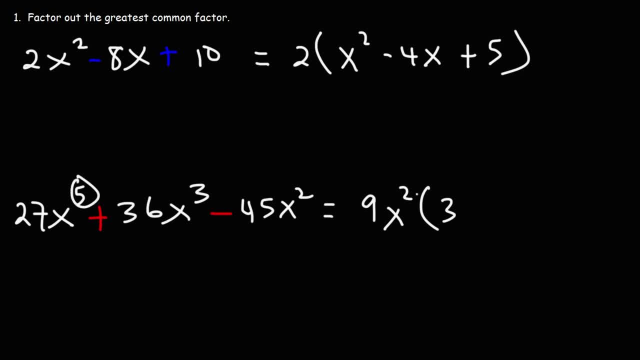 27 divided by 9 is 3.. And then 5 minus 2 is 3.. So we get 3x cubed. Now dividing these two, 36 divided by 9 is 4.. x cubed divided by x squared, or 3 minus 2.. 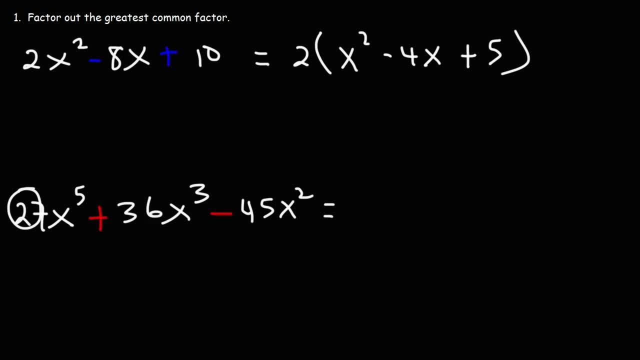 Notice that 27,, 36, and 45,. they're divisible by 9.. And looking at the smaller of these three, it's going to be x squared, So we could factor out 9x, 27x to the 5th, divided by 9x squared. 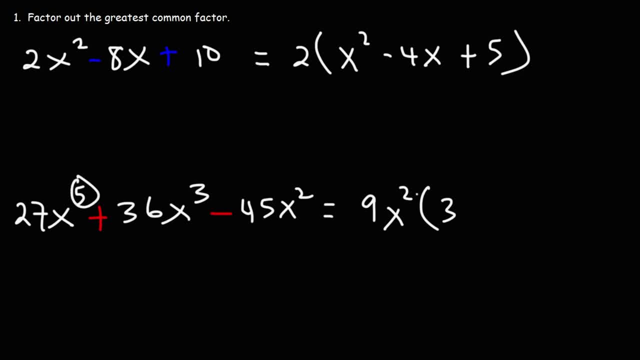 27 divided by 9 is 3.. And then 5 minus 2 is 3.. So we get 3x cubed. Now dividing these two, 36 divided by 9 is 4.. x cubed divided by x squared, or 3 minus 2, that's going to give us 1.. 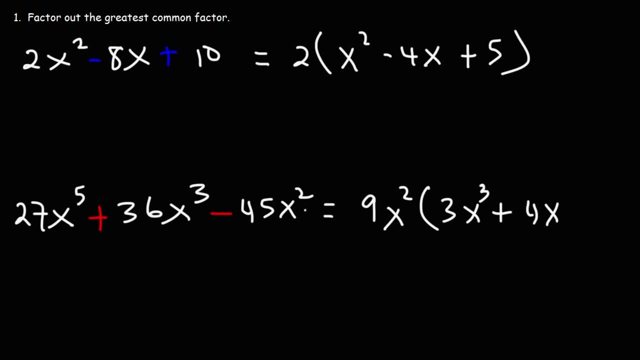 So we'll just have 4x And then negative 45x. x squared divided by 9x squared: Negative 45 divided by 9 is negative 5.. x squared divided by x squared, that's going to be 1.. 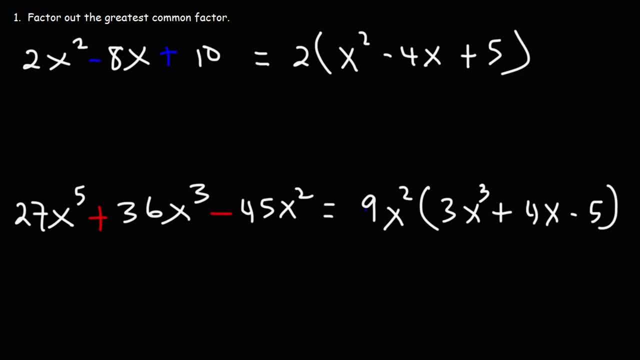 So we just get negative 5.. So this is the answer for the fifth problem. Now, what would you do if you saw an example that looks like this: x times x, x minus 2 plus 3 times x minus 2.. 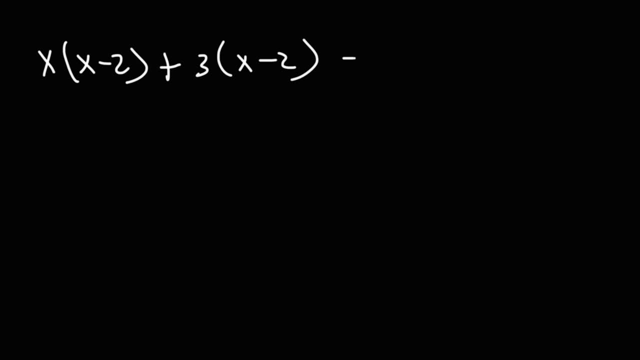 Go ahead and factor out the GCF. Now, the GCF, the greatest common factor is x minus 2.. So when we pull it out, we only need to write it once. Now, if we take this and divide it by x minus 2, what will we get? 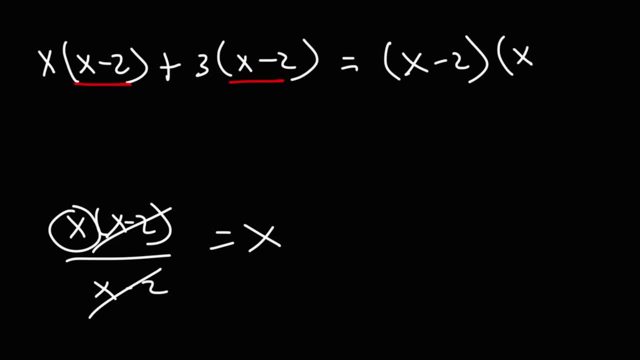 These two will cancel, Given us just x The stuff that we see outside here. The same is true if we divide 3x minus 2 by x minus 2.. These will cancel, leaving behind positive 3.. So that's going to go here. 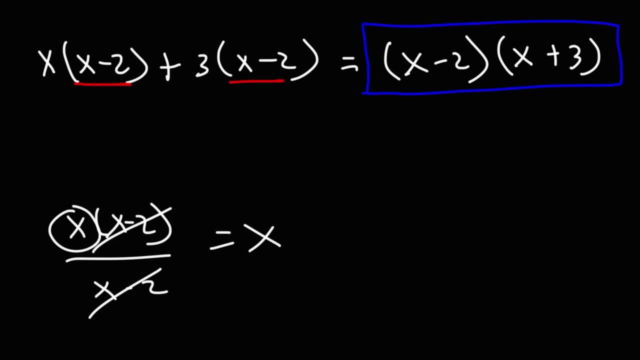 So that's how we can factor out the GCF in this particular example. Now let's try a similar example. This time we're going to have two variables: y times 3x minus 2.. And then minus 4 times 3x minus 2.. 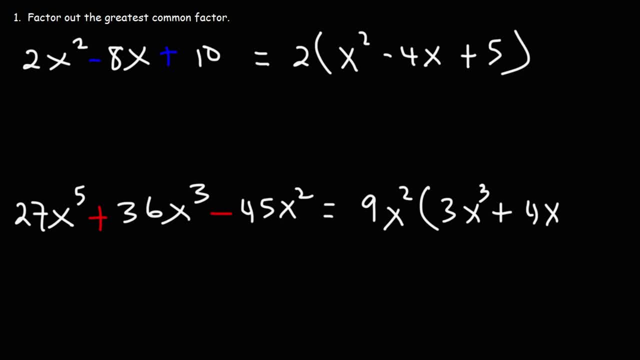 That's going to give us 1, so we'll just have 4x And then negative 45x. x squared divided by 9x squared: Negative 45 divided by 9 is negative 5.. x squared divided by x squared, that's going to be 1.. 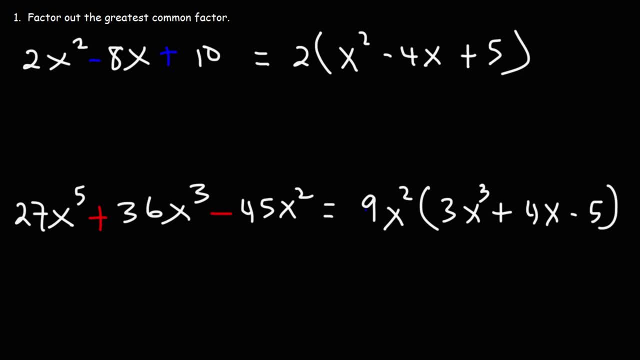 So we just get negative 5.. So this is the answer for the fifth problem. Now, what would you do if you saw an example that looks like this: x times x, x minus 2 plus 3 times x minus 2.. Go ahead and factor out the GCF. 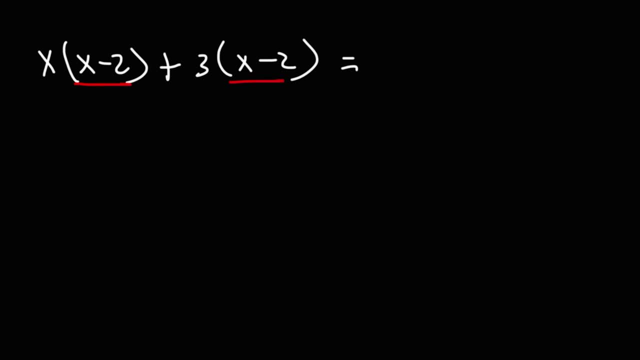 Now the GCF, the greatest common factor is x minus 2.. So when we pull it out, we only need to write it once Now. if we take this and divide it by x minus 2, what will we get? 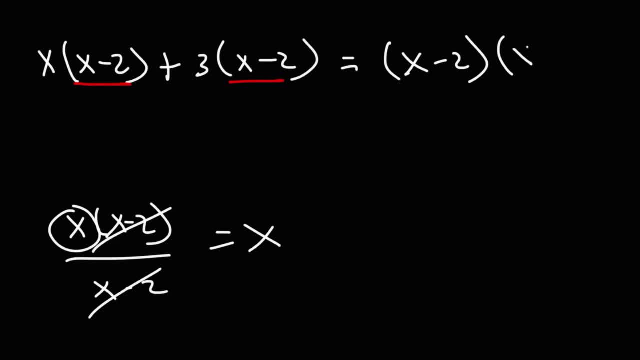 These two will cancel, Given us just x The stuff that we see outside here. The same is true if we divide 3x minus 2 by x minus 2.. These will cancel, leaving behind positive 3.. So that's going to go here. 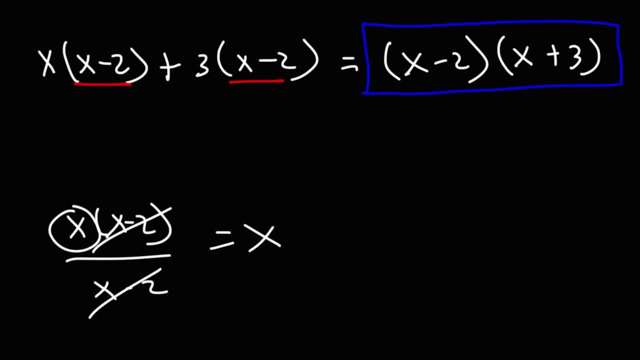 So that's how we can factor out the GCF in this particular example. Now let's try a similar example. This time we're going to have two variables: y times 3x minus 2.. And then minus 4 times 3x minus 2.. 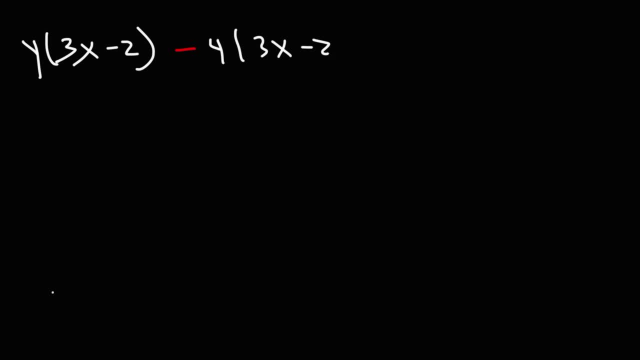 So go ahead and factor out the GCF, So we can clearly see that the GCF is 3x minus 2.. Once we factor out 3x minus 2, we're left with y. And then, once we take it out in the second term, 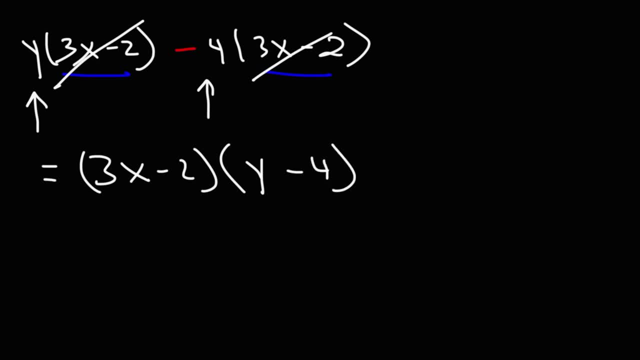 we're left with negative 4.. So the answer is going to be 3x minus 2 times y minus 4.. Now, based on that example, go ahead and try this one. Let's say we have 2x minus 3 times y minus 4, plus 3x plus 8 times y minus 4.. 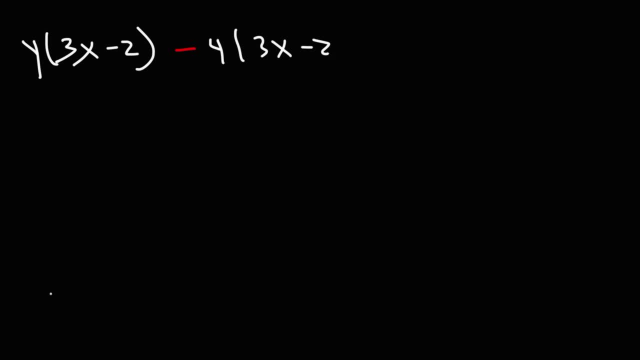 So go ahead and factor out the GCF, So we can clearly see that the GCF is 3x minus 2.. Once we factor out 3x minus 2, we're left with y. And then, once we take it out in the second term, 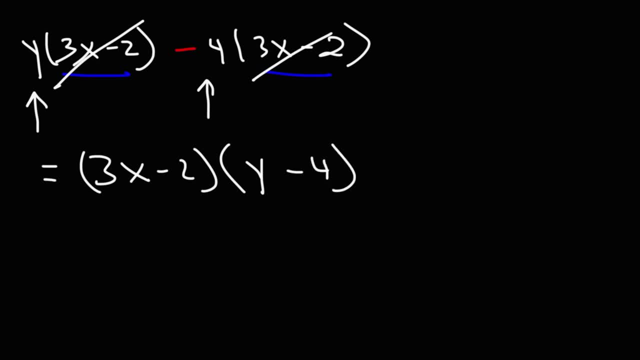 we're left with negative 4.. So the answer is going to be 3x minus 2 times y minus 4.. Now, based on that example, go ahead and try this one. Let's say we have 2x minus 3 times y minus 4, plus 3x plus 8 times y minus 4.. 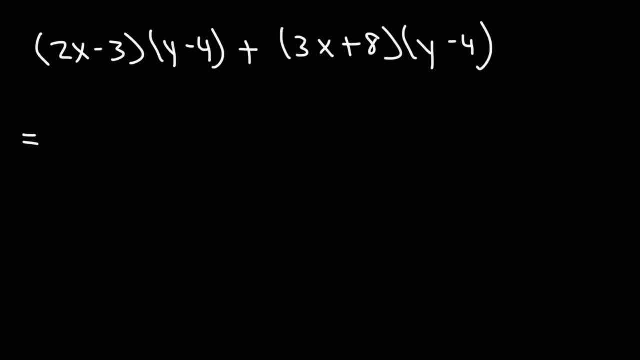 So what is the GCF? in this example? The GCF is the common factor. The common factor is y minus 4.. And it's also the greatest common factor. So if we take out that common factor, what are we going to have left? 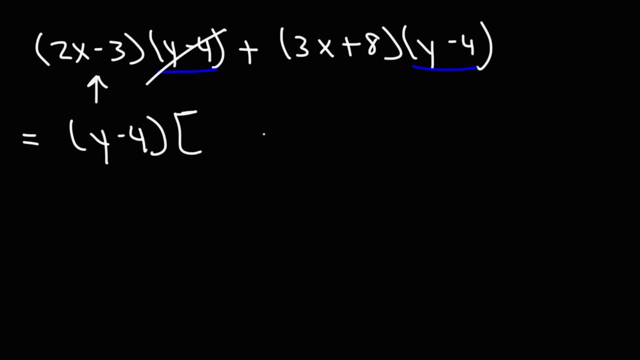 If we factor out y minus 4, we're left with 2x minus 3.. And then we have a plus. Now, if we factor out y minus 4 from the second term, we're left with 3x Plus 8.. 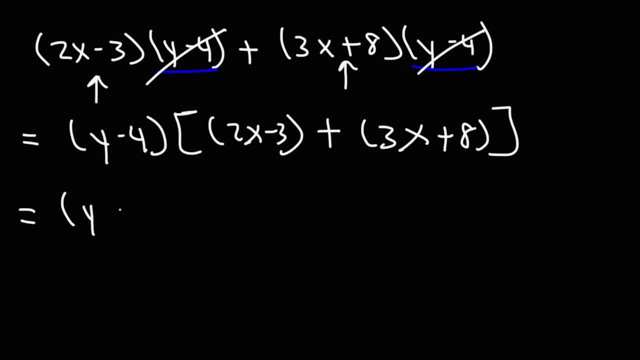 So that's the situation that we now have. So what we need to do at this point is combine like terms: 2x plus 3x. that's going to give us 5x, And then negative 3 plus 8, well, that's going to be positive 5.. 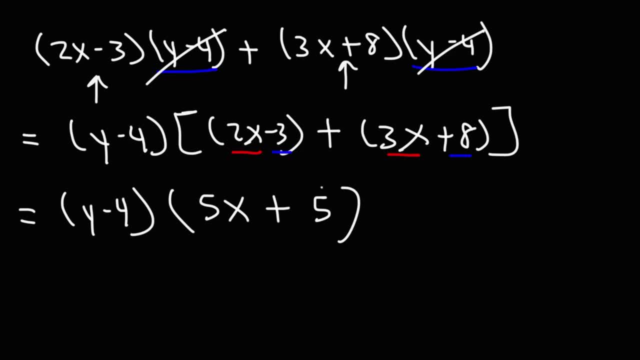 Now we could factor this even further. Here we could take out the GCF, which is 5.. So if we take out 5 from 5x plus 5, 5x divided by 5 is x. 5 divided by 5 is 1.. 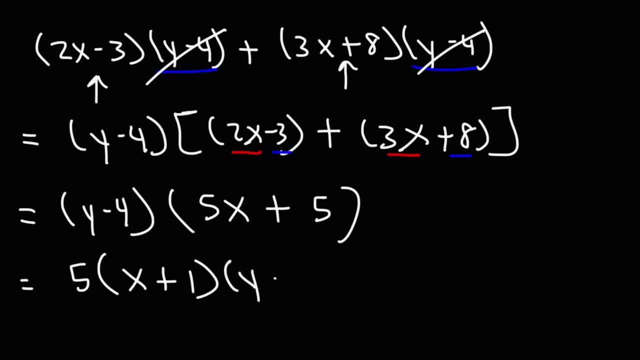 And then we can just rewrite this part. So the final answer for this problem is 5 times x plus 1 times y minus 4..